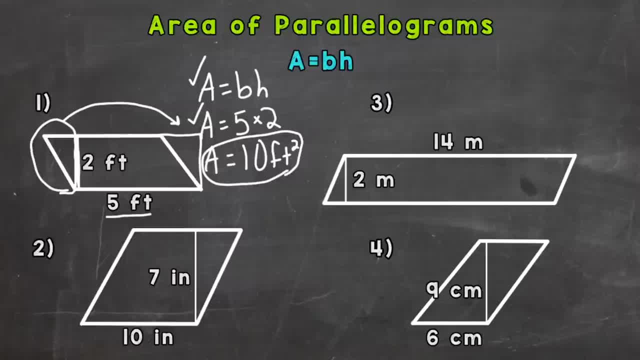 parallelogram. So we're doing the same thing we do with rectangles, And that's why. So, number two, let's write out our formula: Area equals base times height. We will plug in The base, here is the height. And so next, again, Let's add the formula: Area equals base times height. 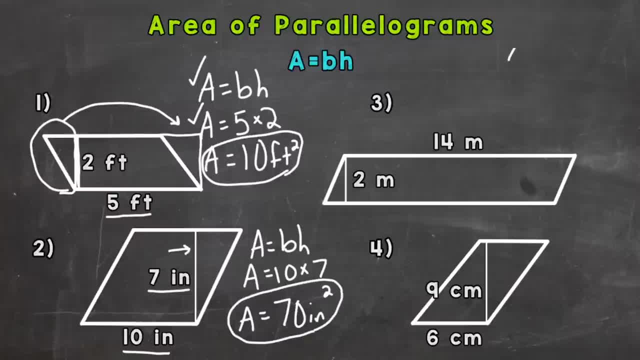 We'll enter into that formula. Area equals base times height. Now what this will do is drive it down a quadrant And maybe a little bit on the obvious side here. Now let's reason and put in a formula here: Area equals base times height. Here is the square size And under span. here this is: square centimeters, And under span here this is a square square. So inside the formula shape is like a circle And under span here this is a circle. So there's an angle, pluswald, And under span that case has maybe four angles, And under span these are Tianca. 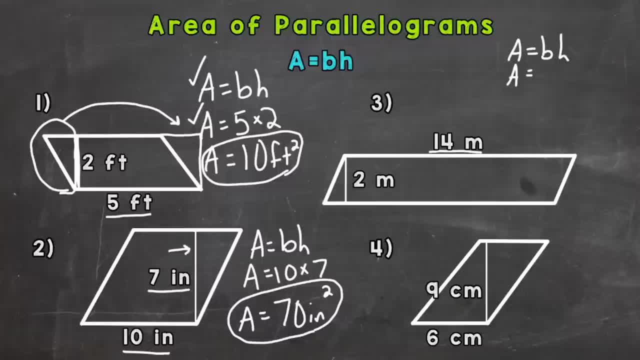 base here is this: 14. it's okay that it's up top the measurement. this bottom side is the same. it's congruent to the top, so it doesn't matter where the measurement is listed. so 14 times a height of 2 and we get an area of 28 square meters and 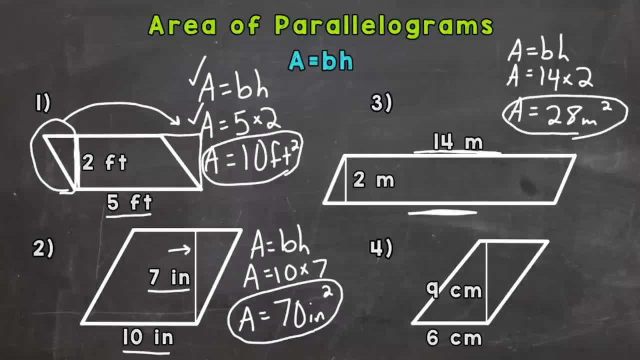 then, lastly, we have a base of 6 centimeters. so let's write out our formula: base times height. plug in our base of 6 times our height of 9 and we get an answer of 54 square centimeters. so there you have it. there's how you find the area of a parallelogram. area equals base times. 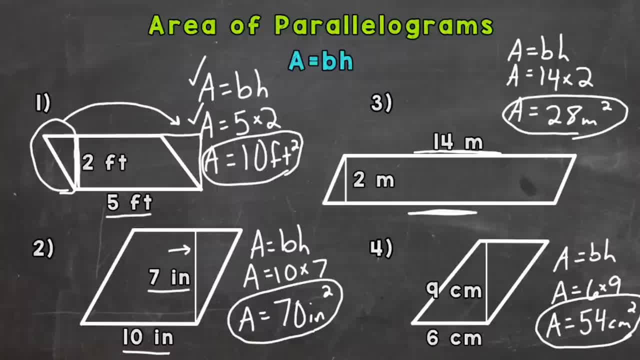 height. and just a reminder, if you take a look at number 3, it works because if we take a portion of our parallelogram and move it to the other side, it'll actually give us a rectangle. that line doesn't perfectly line up, but hopefully you kind of see the point there where I'm going with things. so 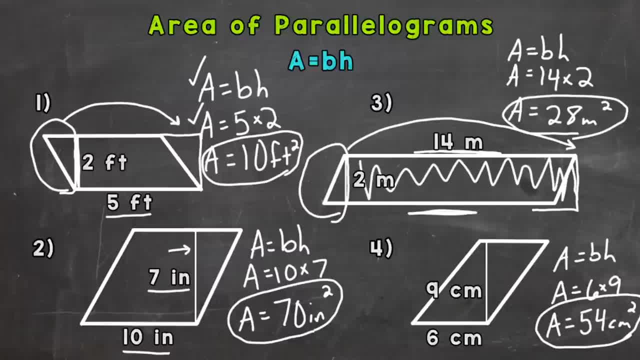 this would be our rectangle here, okay, so hopefully that helped. thanks so much for watching. until next time, peace.